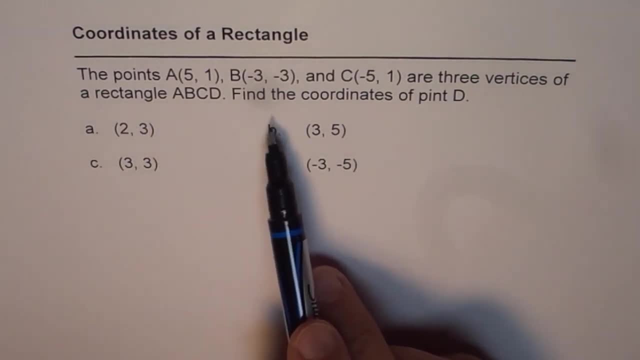 of a rectangle: A, B, C, D. Find the coordinates of point D right. So P O I and T point D. So that's the question: How are you going to do it? Well, there are many ways you can do it. 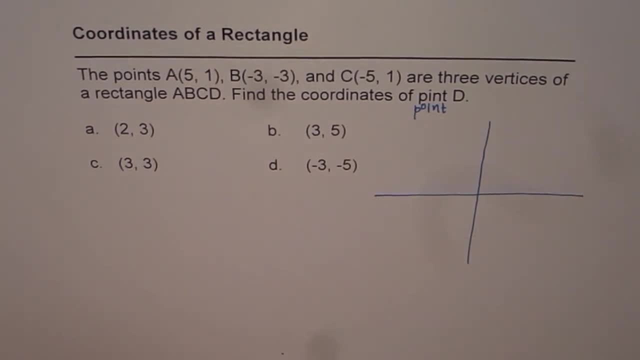 but here is a very simple way of doing it. Just to explain you, let me plot these points approximately on a Cartesian plane. We say A is 5, 1.. So let us say this is somewhere here 5, 1, and let me say this is my point A, which is 5, 1.. Point B is minus 3, minus 3.. So 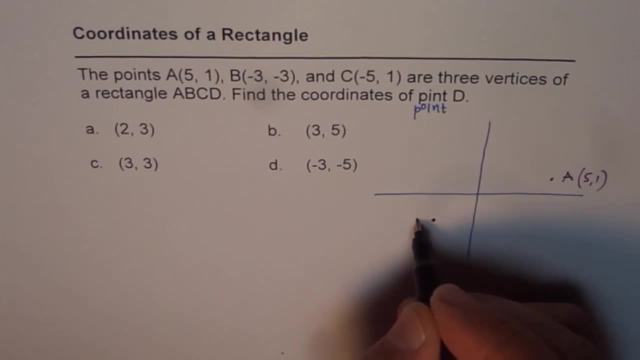 that is approximately. let us say, this point is point B for me, which is minus 3, minus 3.. C is minus 5 and 1. So let's say 5 and 1.. Okay, so almost at the same line. there we have minus 5. 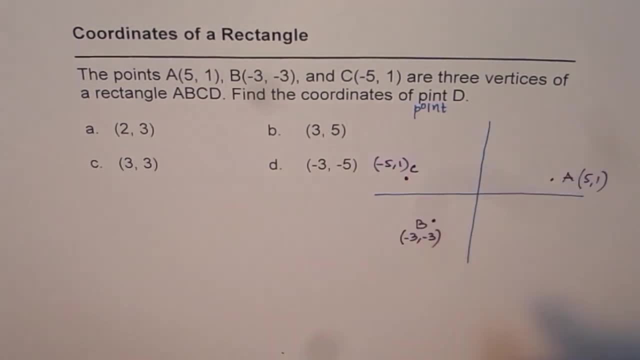 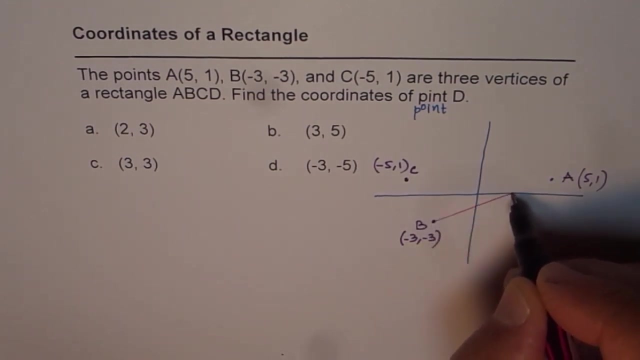 and 1, and this is point C for us. Now we need to find where point D is. So that is what the question is. How will you do it? Well, let me first connect these, just to give you an idea. How should we? 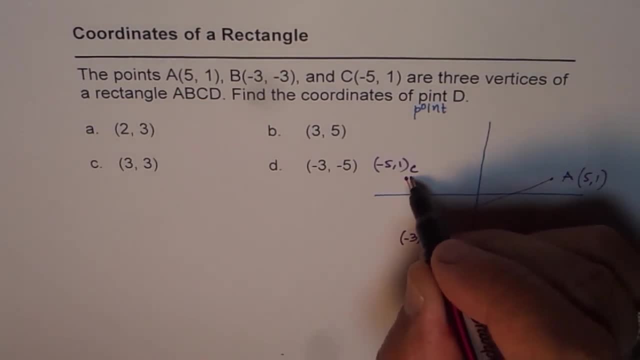 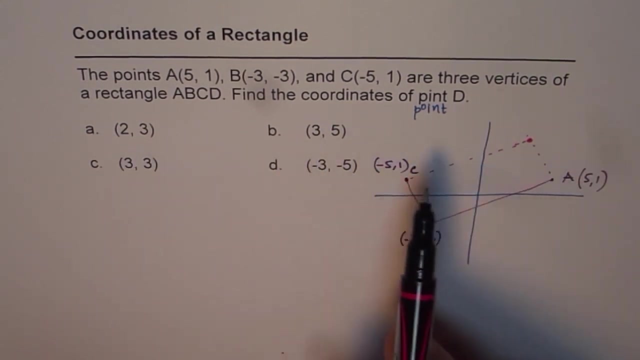 be going about. So obviously that point is somewhere here. a line parallel to AB and then a line parallel to BC should make us give us the point right. 3. Well, from the multiple choice questions we can rule out the last one. Any of these could be possible. 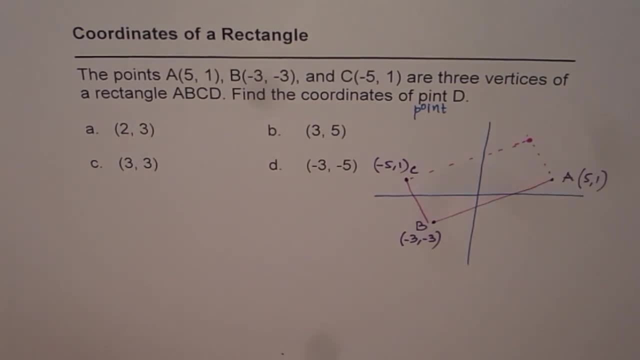 How? How do we get that point? That is really the question. Now, easy way is to find: how do we get A from B. So if I am going from B to A, then if I am here at minus 3 and I want 5, what do I do? 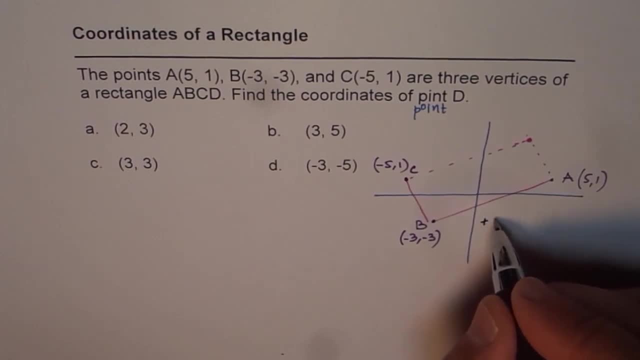 Do X values. I will add 8 to X values. right. So to X values. if I add 8 from minus 3, I get 5.. Now, how do I get the Y value of 1?? Now, to get the Y value of 1 from minus 3, I have.